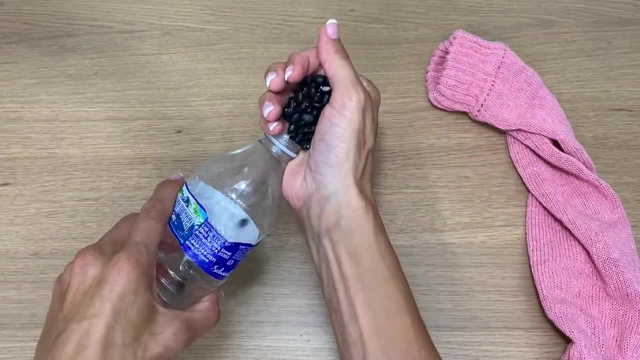 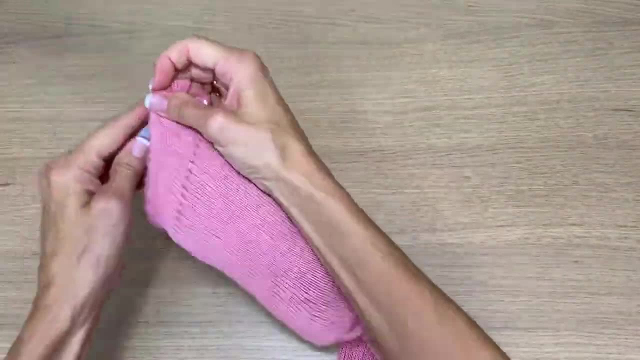 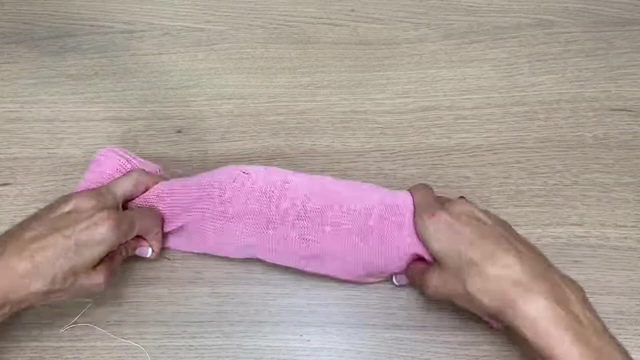 You can use also a longer sock and rocks instead of beans, Just in case you don't have any of these things here, And if your sock or leg warmer is long enough, you could just tie the ends. Mine weren't, so I just used a needle and thread to really secure the sides. 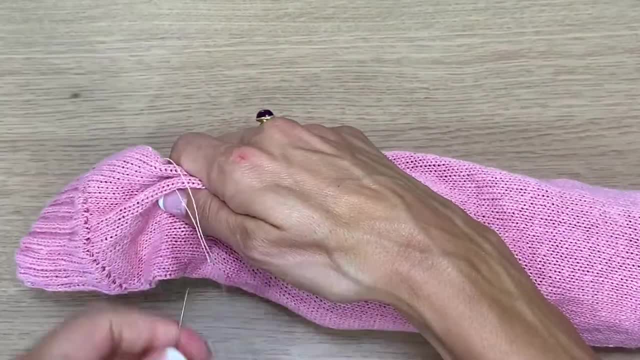 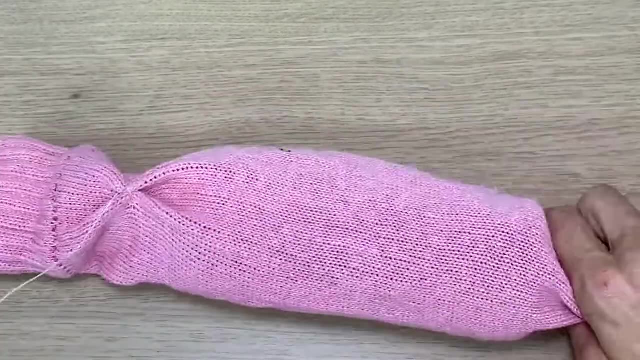 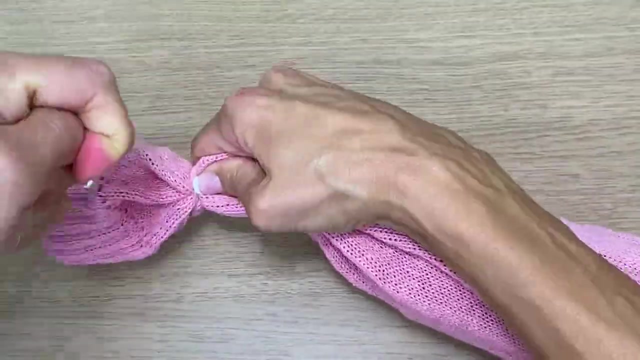 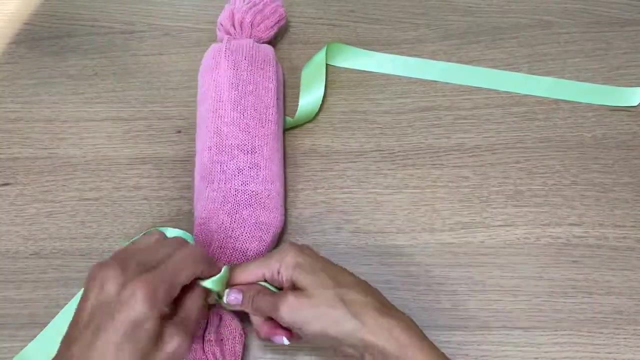 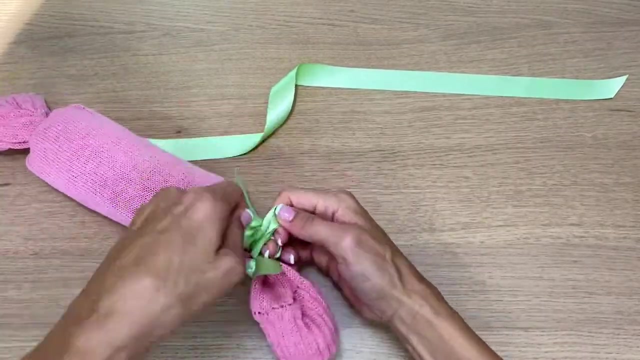 And it kind of looks like a long fitzy roll Rolled up here, Loving this tutorial. Please subscribe so you can stay up to date with all my latest videos. I'll see you next time, Take care, Bye-bye, Goodbye. 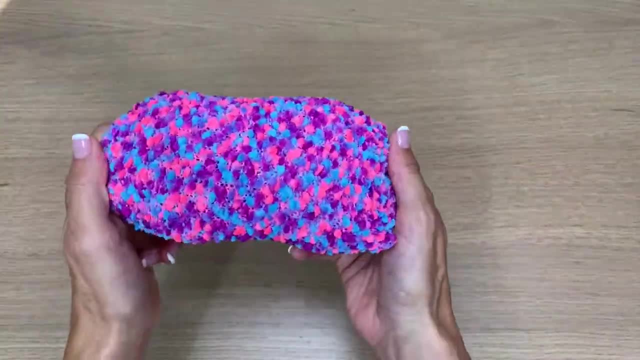 And that's it. How easy was that. So next I'm going to show you this crinkled plush. Again, another sock from my Dollar Tree, And that's just a plastic bag that I don't know. I eat it once in a while. 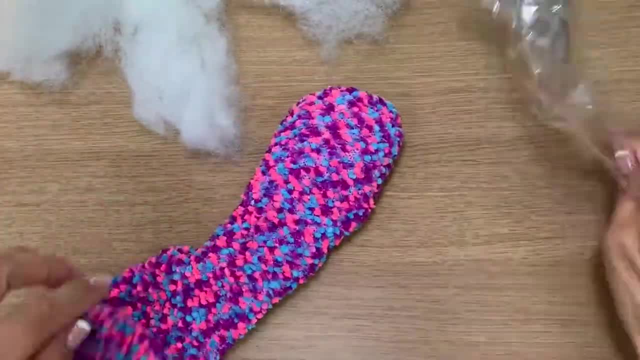 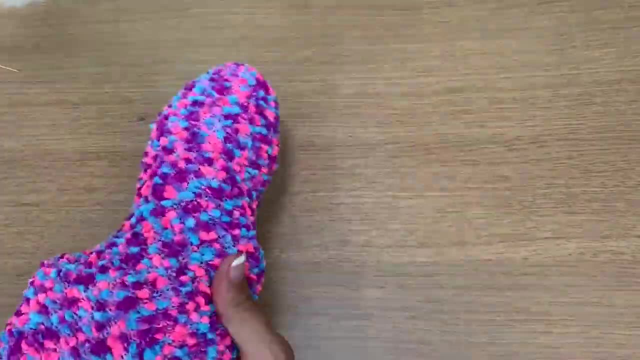 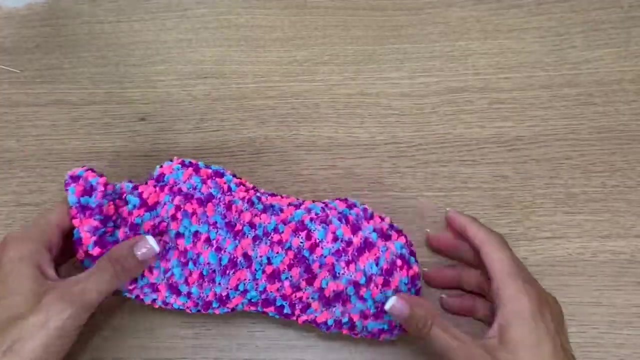 ordered something from amazon and it was wrapped in that bag and i like the sound of it. so here we go, a little stuffing stuff, the bag in there as well, and then a little bit more stuffing in there. then i am going to turn this open end of the sock into the plush, just like this. 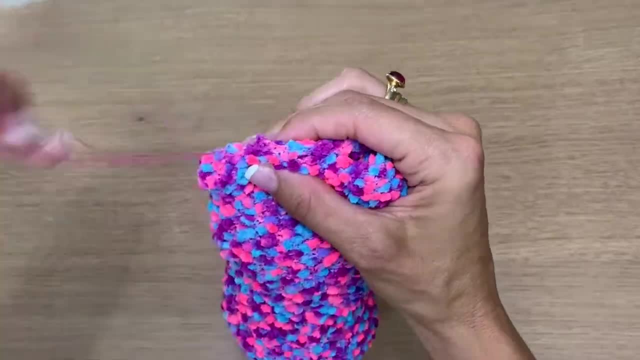 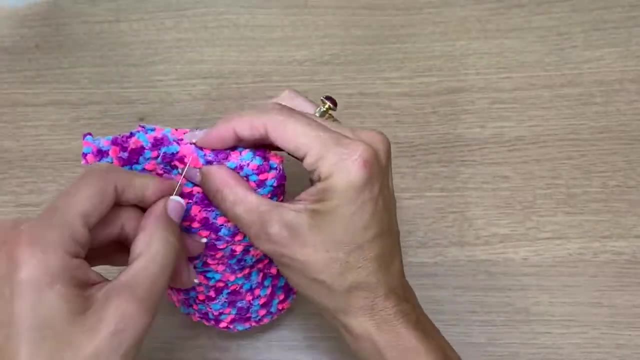 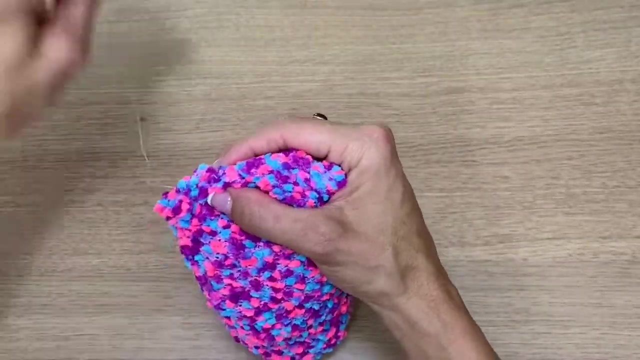 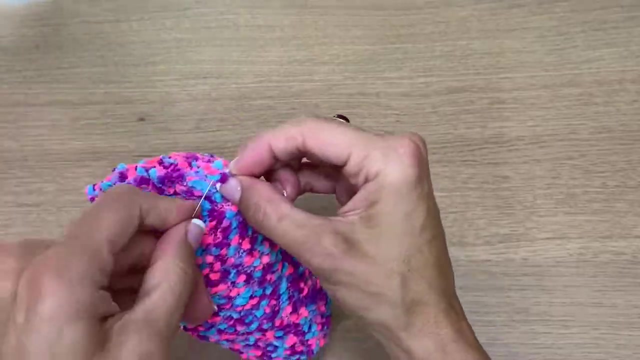 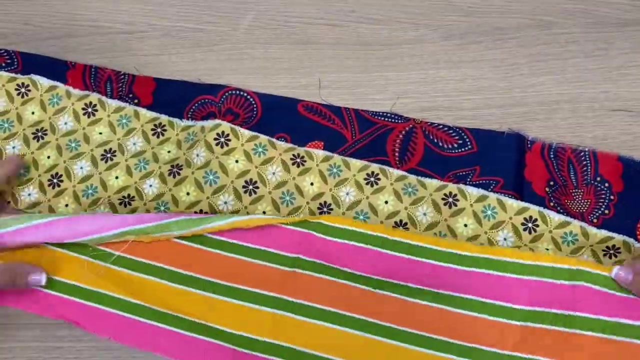 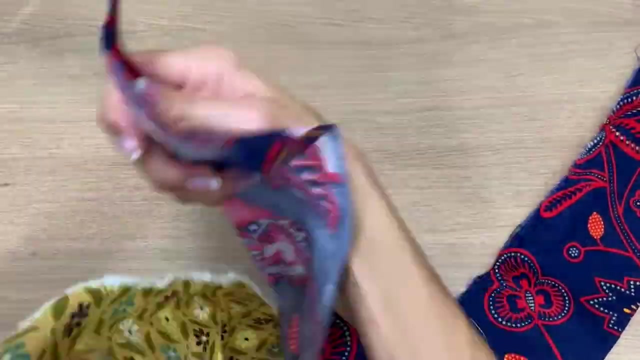 and then with a double threaded needle, with coordinating thread. i'm just going to give a little closure there with a simple overcast stitch. and now i'm going to show you how to make this tug toy that's braided, so i'm using scrap fabric. You can cut it as long and as wide as you want. You can even if you don't. 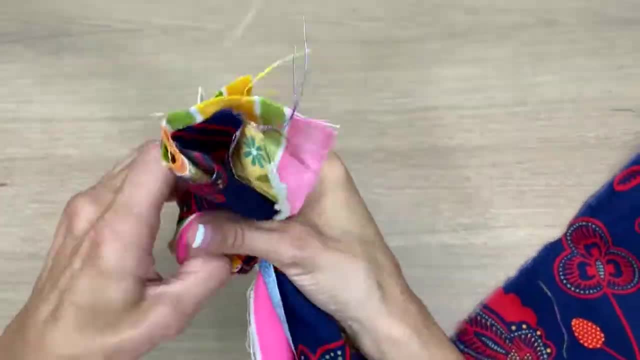 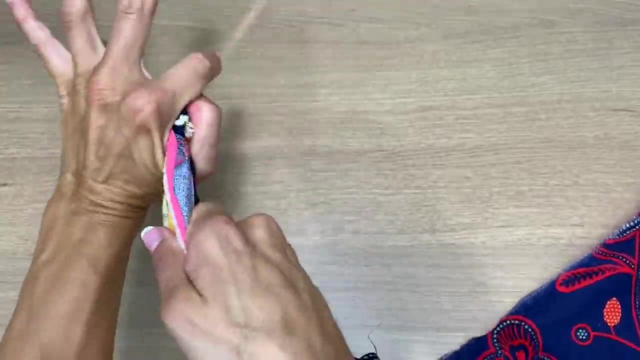 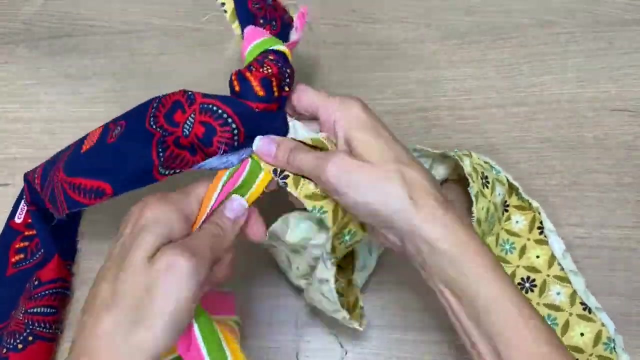 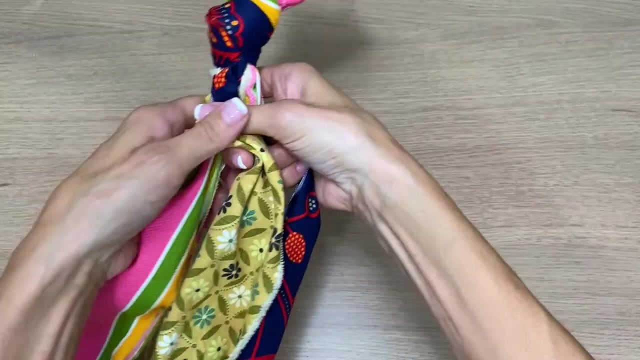 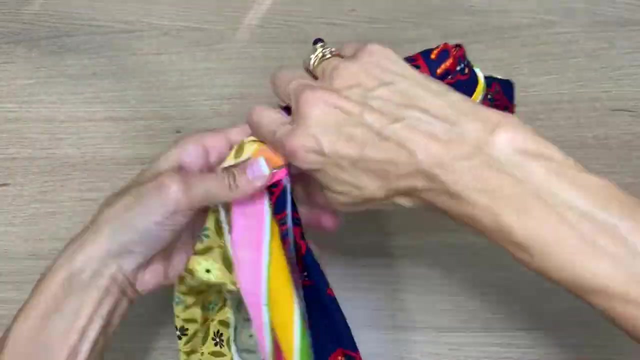 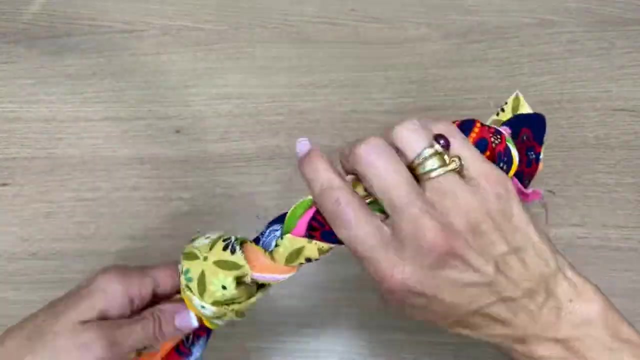 have scrap fabric, use jeans, clothing, anything you have that's long. You're going to tie one knot at the end and then you're going to pull that really tight and then you're going to braid your strips of fabric And as I reached the certain length of braiding I made a knot. I just had all three strips.